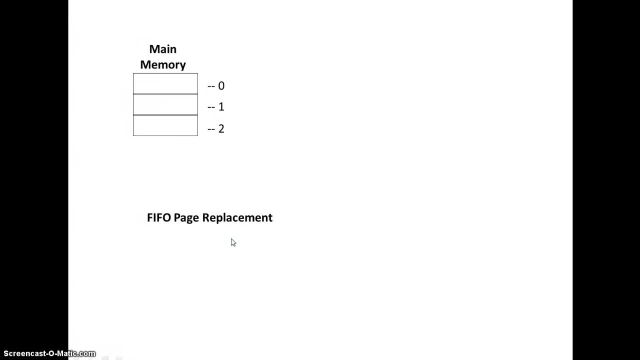 Now just showing it this way. one of the things that we miss if we're trying to follow is sort of a record of where we were at a point in time, meaning, suppose that the first thing we need to do is reference page A? 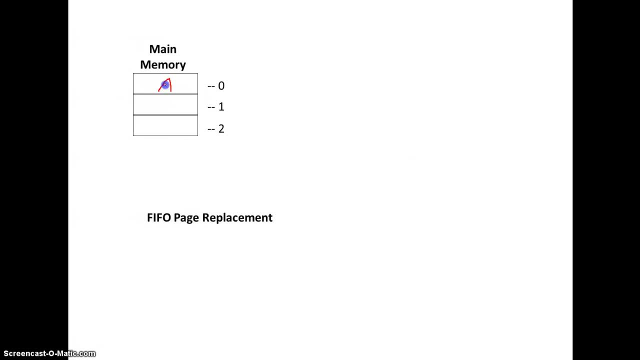 Page A is not in memory, so page A is brought into memory and is here. Then we need to reference page B. Well, page B isn't here, so we have this empty page and the page B is loaded here. We need to reference page A. Well, page A is here. We need to reference page C: It's not here, and so we have this free place. 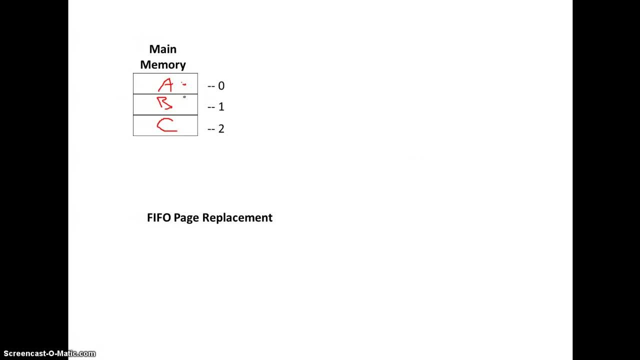 And it's in memory. We need to reference page A. Here it is. We need to reference page B: Here it is. We need to reference page D. It's not here. So now we need to take one of the pages out, And first in, first out, we would take the oldest one, which in this case is the A, and now replace it with this page D that we reference. 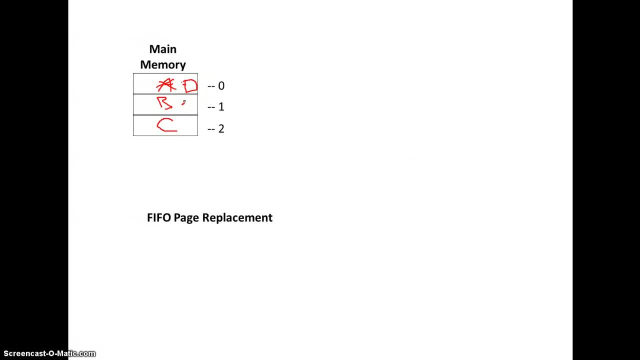 We're now looking for B, which is here. We're now looking for A, which isn't, so. we have to take the oldest page first in, first out the oldest one, which is this B. This B is now becoming A, And now the next page reference is B. Well, B is not in memory, so we have to take the oldest one. 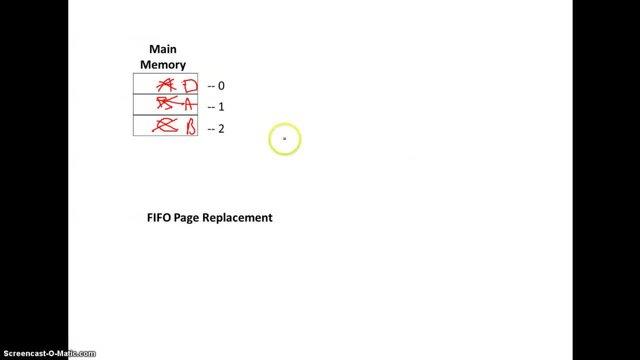 which in this case now is this one, and replace it here with B. Now, I know I went pretty darn quick and I was trying to illustrate a point is that, yeah, I got through up to this point and this is how memory looks after all of those page references are done. but I have no way of kind of looking back at the history to see, uh, 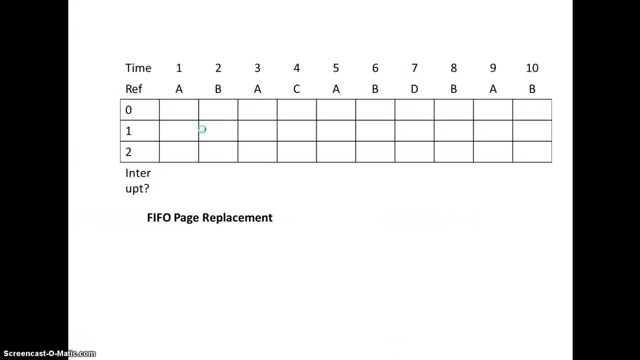 But I have no way of kind of looking back at the history to see, uh, what we're doing here, But I have no way of kind of looking back at the history to see, uh, what happened. And so that's why what the book will introduce to us is this page reference table. 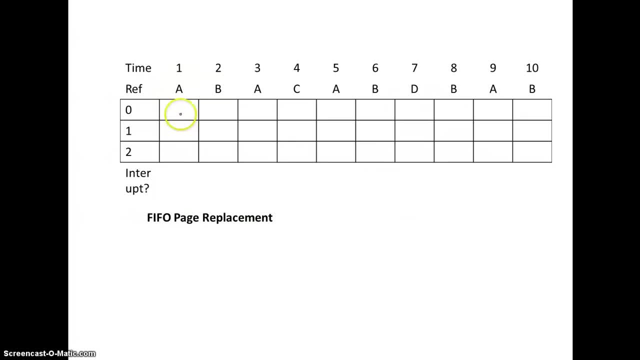 And? um, so, if we have only three frames that we're dealing with, that's why we're showing here, uh, our three frames: 0 and 1, 2.. Um then, what this here is representing is the page that we are looking for. 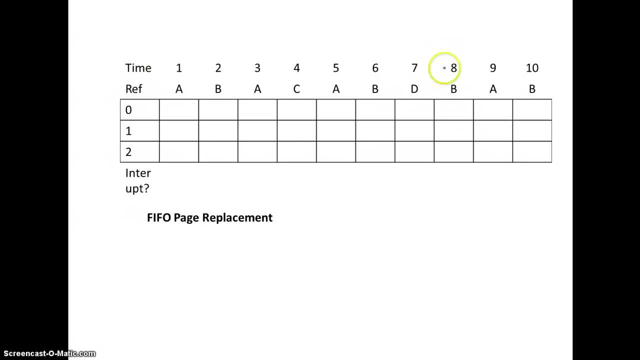 Um, here we're showing time that's increasing. These are just 10 steps, uh, over time, And the other thing we can keep track of is whether or not uh an interrupt occurred, meaning, uh, did it have to do anything to bring that page uh into memory? 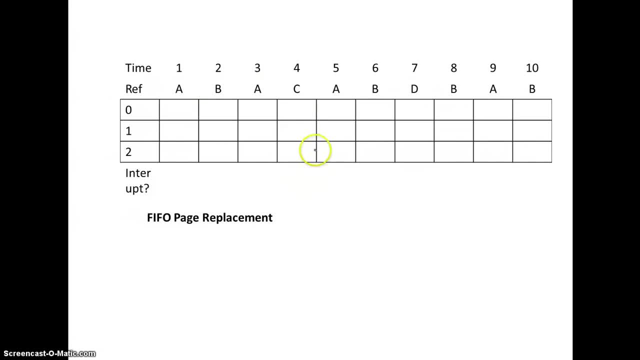 Um, and so what'll happen is, as we advance and fill the table left to right, uh, it's the kind of thing we can look back and see what happened at any point in time. Um, so, even though- let me just back up a second, even though memory only has these three frames- 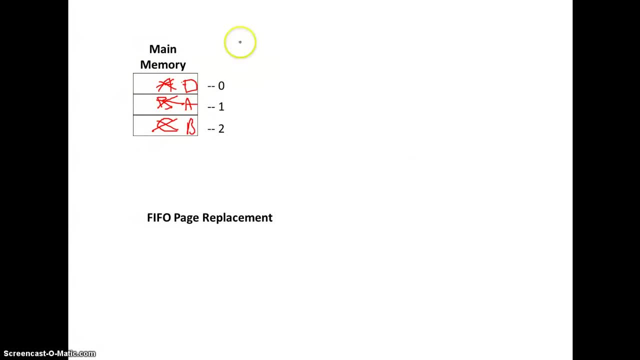 as you saw, you know I was replacing the the different frames, what I have right here. there's no way of history to see what happened Um, so here what I can do is um keep track of the history. 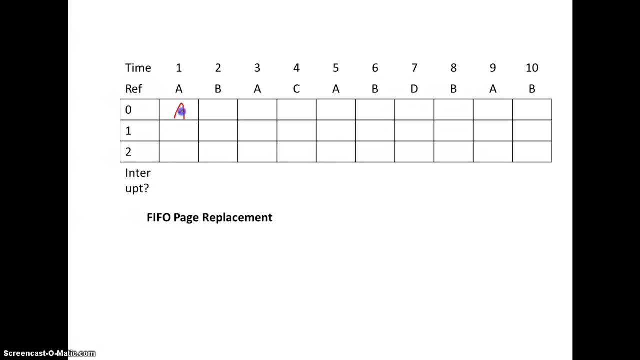 So we go to refer to page A. It's not here. So we have, uh, page A And we took an interrupt to actually go and and bring that page in. Now, the next point in time, we go to reference B. 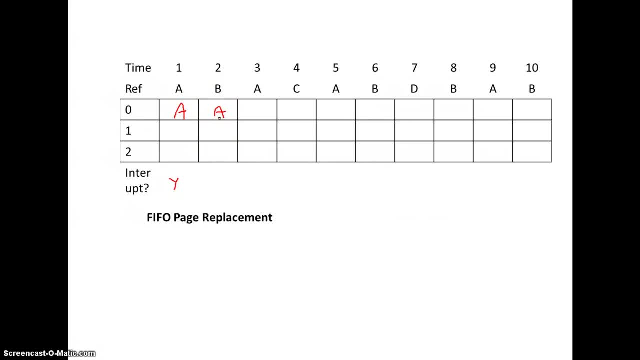 Well, A is already in memory. That was already there, Remember we? we just begin by sort of making a copy of what was there. uh to here. So we're basically saying at timeframe 2, this is what memory looks like. 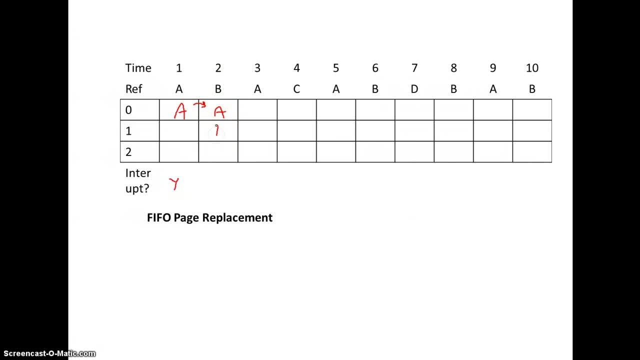 And we're trying to reference B And uh, B is not there And so we take the hit to bring that in. Uh, the next point in time. well, how our memory begins. before this next page reference, it's beginning looking like this: 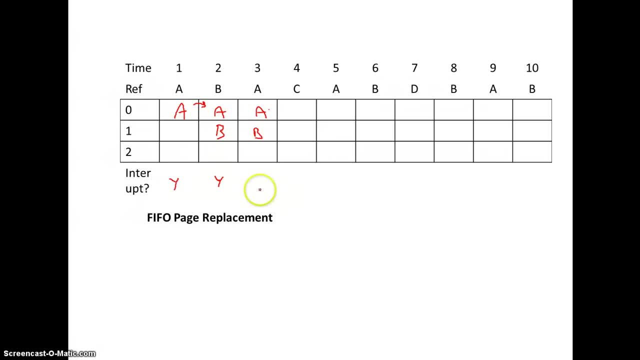 Now we're referring to A. A is already here, So we're not doing uh, uh, an interrupt, Um, the next point in time. so here our memory is looking like this: our A and our B, And now we're referring to page reference C. 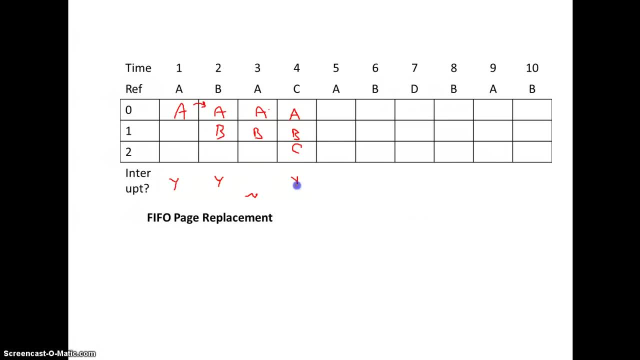 C is not in memory, And so we're taking interrupt. uh for that Um. now we're looking for page A, Um. so first, this is what our memory is looking like at the present moment: our A, B, C. 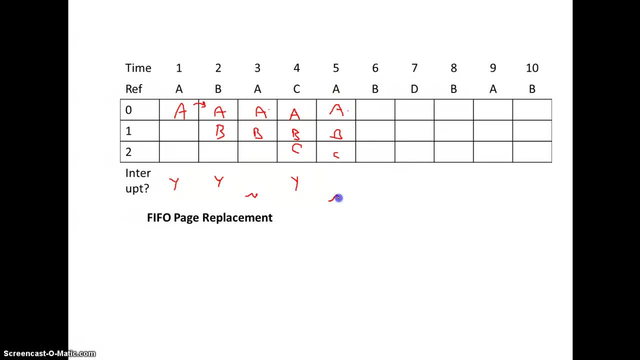 Uh, we're looking for page A. It is in memory, So this is not uh an interrupt. Um, we're looking for page uh, memory. Uh, B, Um. again, this is what our memory looks like at the present moment. 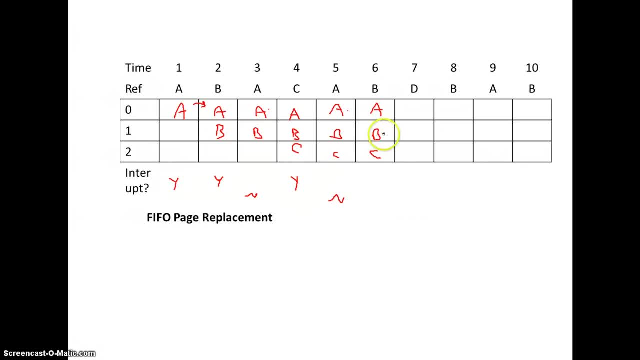 Um, our B is in memory. Okay, so there's not an interrupt for that. Now we're looking for page D. Well, at the present moment, before we look for the page D, this is what memory looks like: That we have page A, page B, page C. 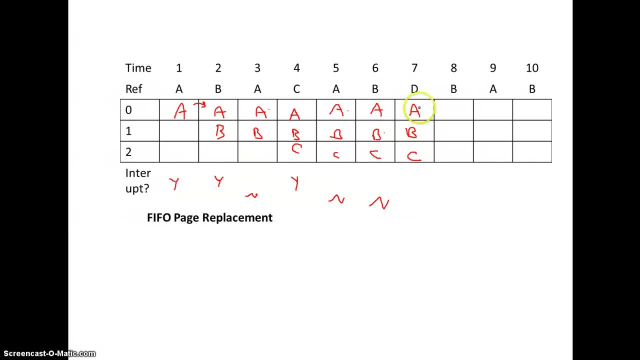 Well, page D is not in memory, So this is when, um, uh, the operating system wants to figure out if we're using first in, first out. uh, the oldest page that is here And the oldest page, the one that's been here the longest, is A. 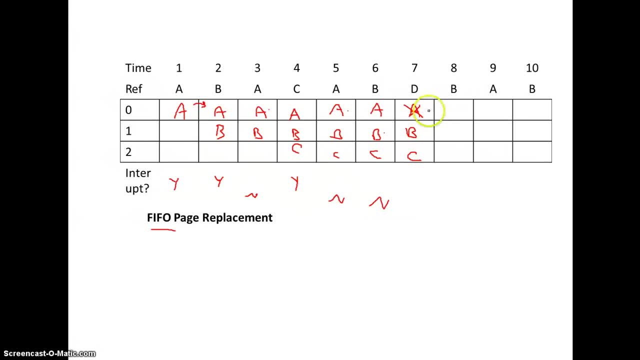 So A is the one that is going to get replaced with page D, So with the first in, first out is when a page needs to be replaced, It is replaced with the oldest one at that point in time. So now our next page reference. well, our memory at the present moment. 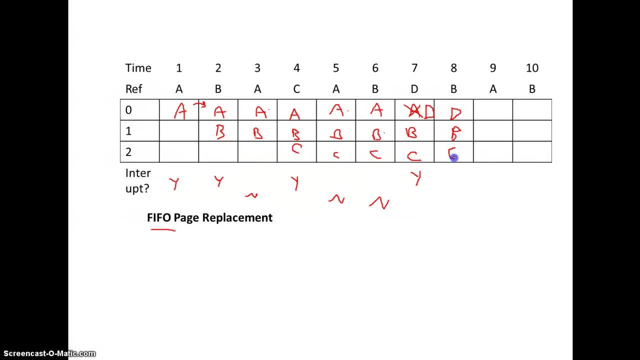 looks like this: or D, B, C, And we're referencing B, but B already is in memory, So we're not doing an interrupt for that Um. now here for the next reference. we're referencing page A, Um. page A is not in memory. 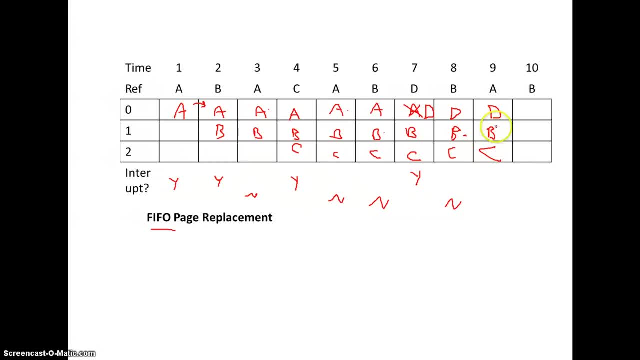 So then we take, of the pages that are here, the D, B and the C. the one that has been in memory the longest is the B, So this is the one that is going to be replaced with A, And we did take, uh, an interrupt for that. 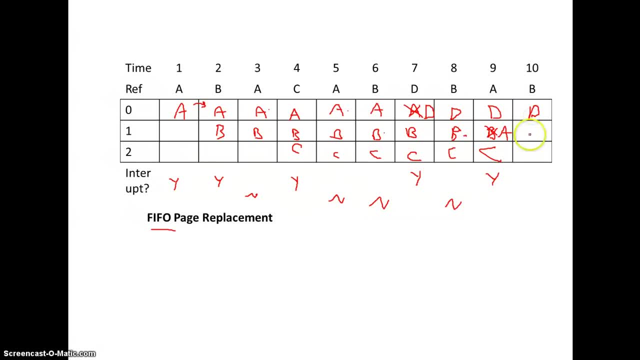 So now we do a page reference. Currently our memory looks like this: B is not, this is a D. I'm sorry if you're looking, I'm just copying over. This is just. I got lousy handwriting when I use- uh, the mouse. 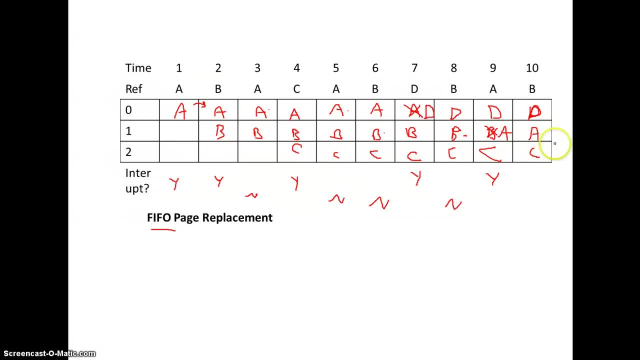 B is not in memory, So now the operating system has to take the one, that of these pages that's been in memory the longest, and that is uh C, And so this is being replaced now um with B. So what we now have by using this page reference table. 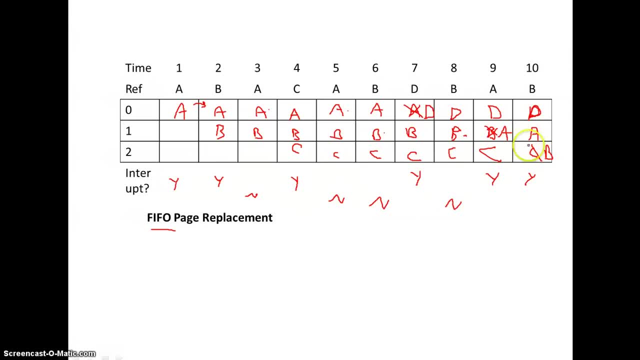 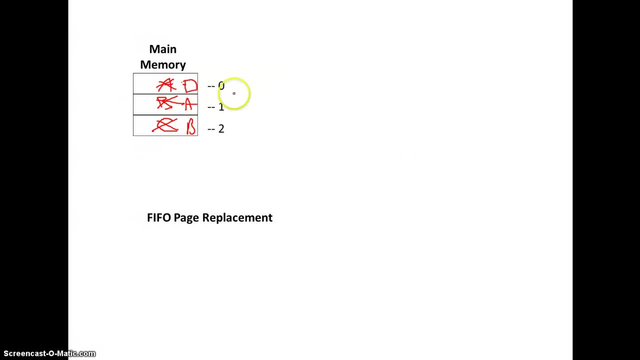 is, although, in terms of the current moment in time, we're seeing here the D A B which, if we look back, that is how we ended up over here. uh, the D A B. Um, what we're able to do is.